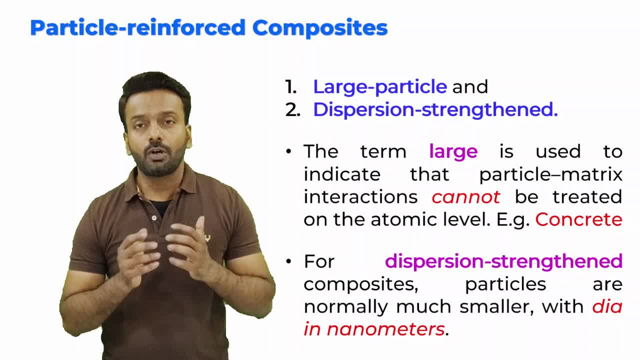 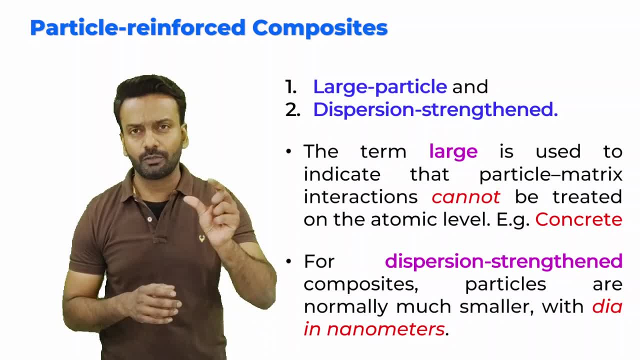 For example, as we have seen in an earlier video, concrete. So concrete is a combination of large gravel, So these are not at an atomic level, They are macroscopic, So we can see them with our naked eye. That is why they are called large particles. So why they are called large particles? because we 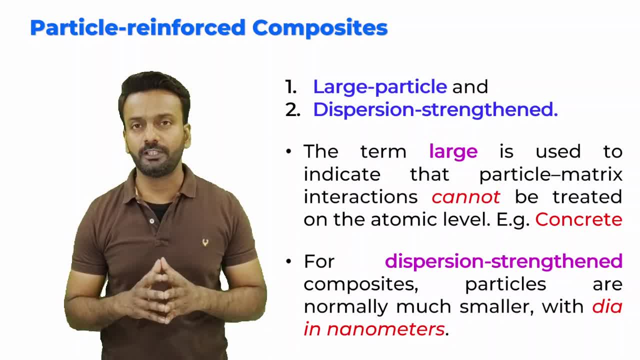 call them as large particle- reinforced composite material. On the other hand, we have dispersed particles. So here these dispersed particles are at an atomic level, Mainly they are at a nano scale. That is why we call them as dispersed particle- strengthened composite materials. 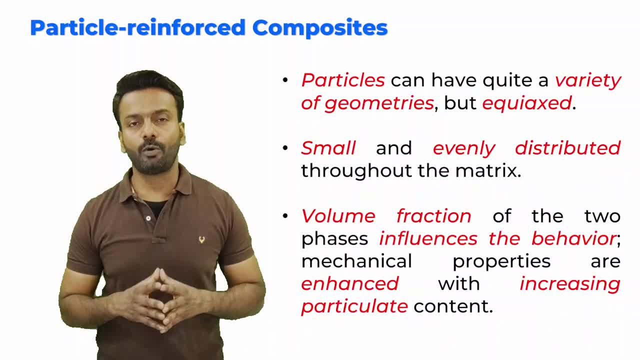 In particle reinforced composite. the particle can have a variety of geometry, but they are supposed to be equiaxed. They can be small and they can be evenly distributed throughout the matrix. Here the volume fraction plays a very important role in influencing the final properties of the composite. 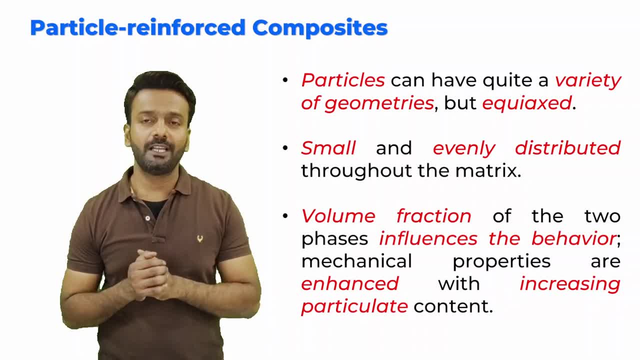 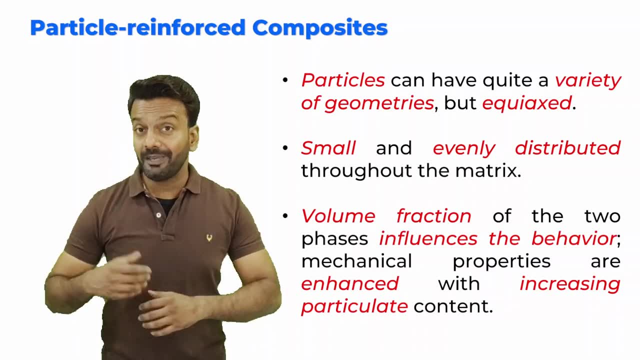 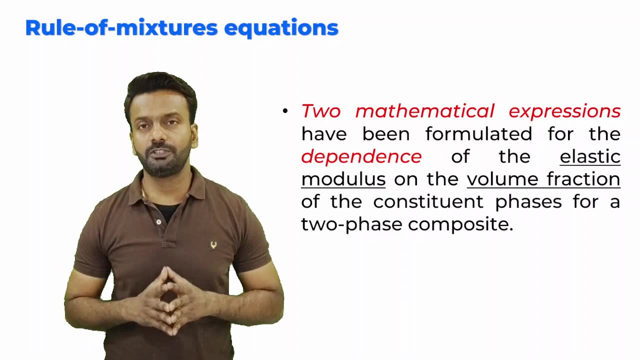 material as well as the mechanical property, are influenced by these small, small particles which are there. As we increase the volume, fraction of these particulate matter, the mechanical properties are also enhanced. Rule of mixture equation. So what is the rule of mixture equation Here? two. 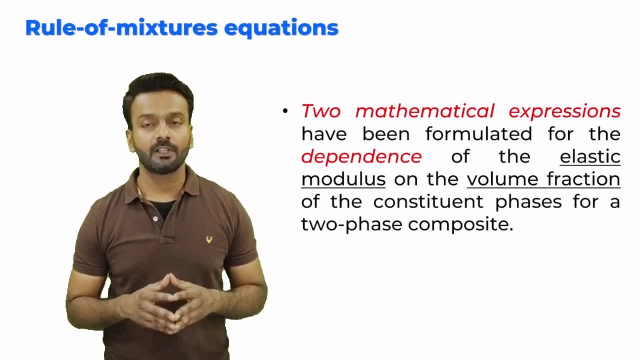 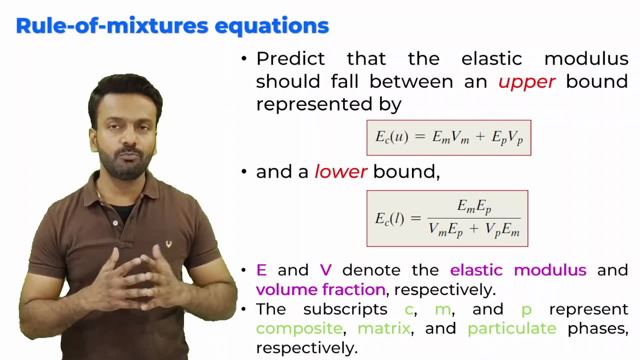 formulas have been derived which are used to calculate the final property of the composite material, Based on elastic modulus and volume fraction. together, both of them influence the final property of the composite material. So these equations, they predict the upper limit and the lower limit of the elastic modulus of the composite. 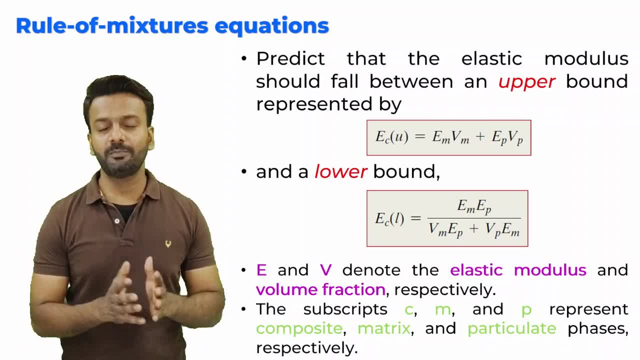 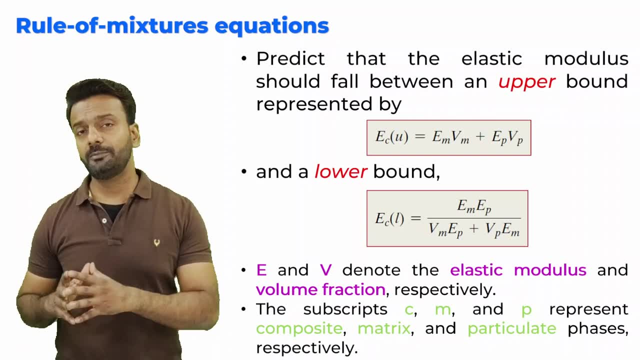 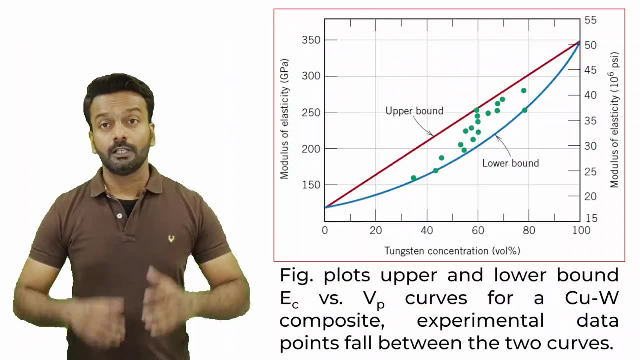 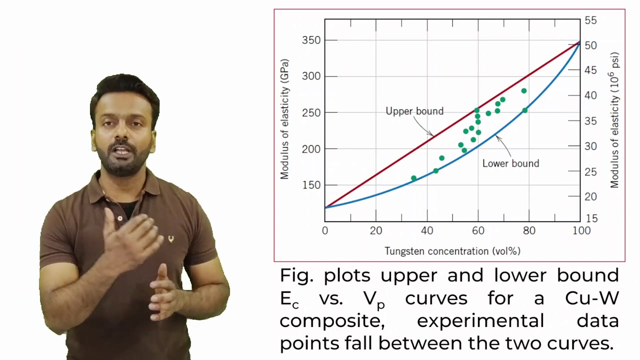 material based on the volume fraction. Here E and V represent the elastic modulus and volume fraction respectively. C, M and P represent composite material And the matrix material phases respectively. This plot shows the upper bound and the lower bound limit of a proper tungsten composite material. So the upper bound and the lower 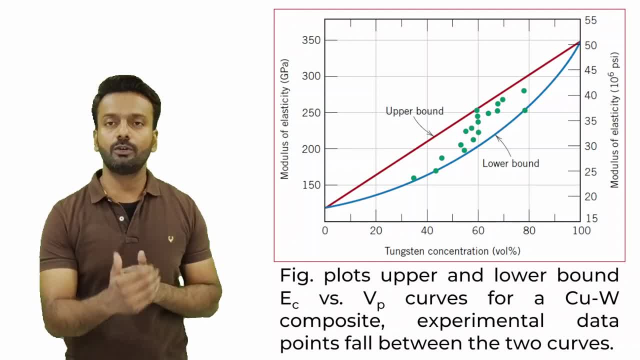 bound limit based on the calculation of the formula, is drawn or plotted on this figure And the dots which you see represent the actual experimental data which exactly falls between the upper bound and the lower bound limit. So we can say that we can easily predict the property of the. 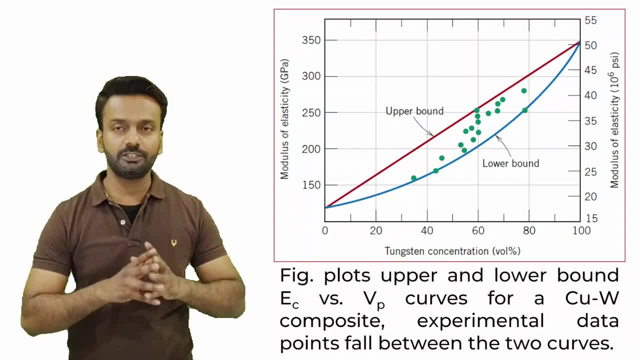 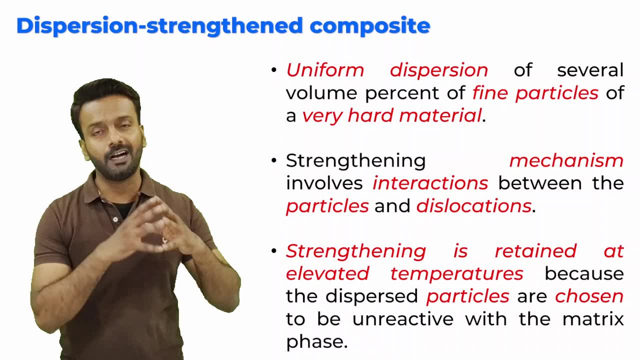 material based on the rule of mixture formula or equation In dispersion. strengthened composite material. several small particle of the dispersed matrix are there in the composite material and these small, small particles are very hard in nature. That means their strength is more hard than the matrix material. So the strengthening is happening mainly because of the interaction of 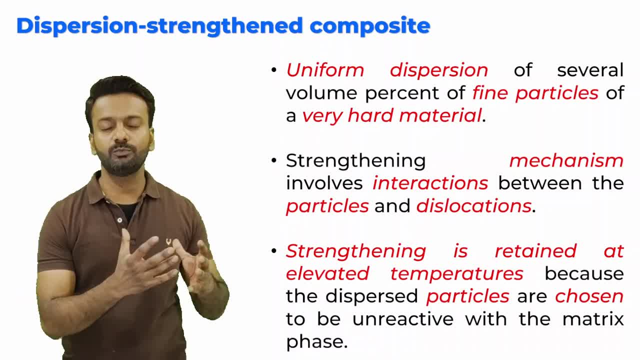 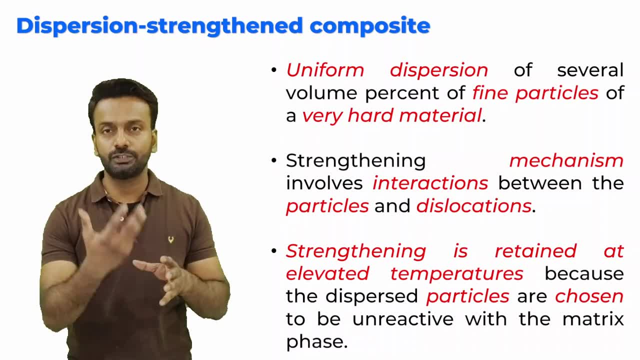 these particle and the dislocation. So when the dislocation is moving along, when there is a plastic deformation, these dislocation will encounter these particles or these particle phases which are stronger, and the particle phase will ping the dislocation. So the dislocation cannot move further. 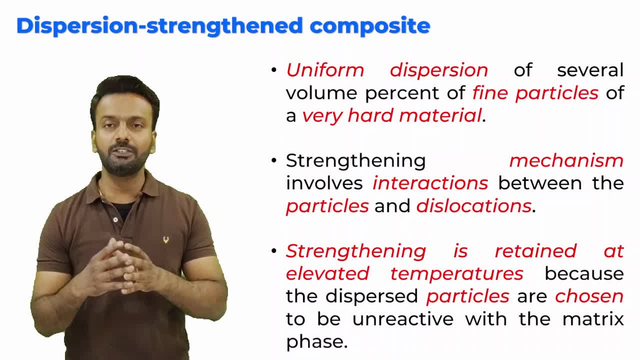 So you will need some extra strength to be applied externally so that the dislocation can move further and you get more plastic deformation. So in totality, it appears that the material is more stronger when you are applying more force, So when the dispersed particles are there throughout the 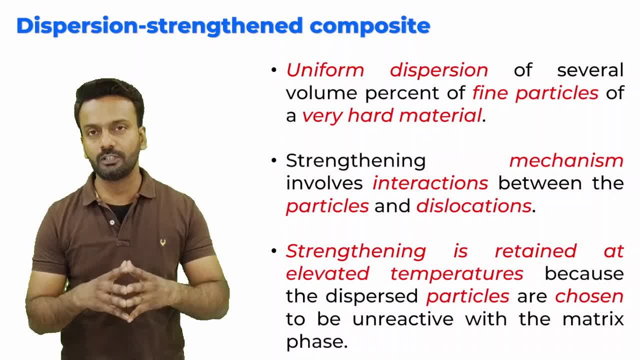 matrix it will appear that the material is more stronger And when the dispersed particles are there, it will also give the expression or expression of the heat of the material. These kat, Ε and Kδ are three huge particles. the material has become more stronger. one more important point: the strengthening can be retained. 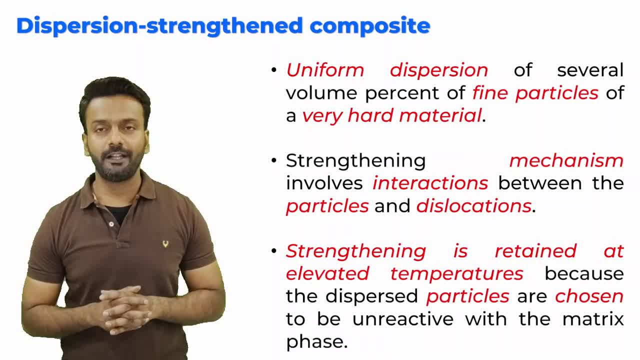 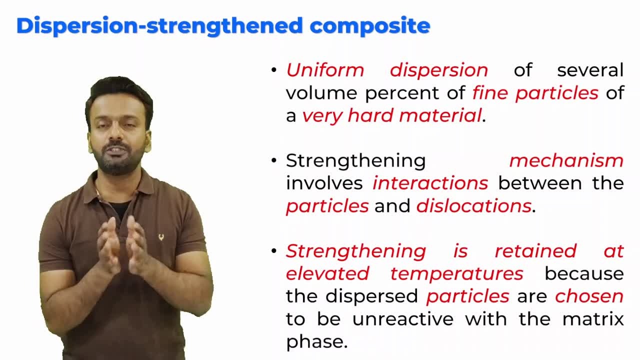 at an elevated temperature because you are selecting the particle phase and you know, based on your application. suppose you want something to be operated at an elevated temperature, so the dispersed particle will retain that strength at an elevated temperature and you are choosing these dispersed particles based on these properties which they are having. so they 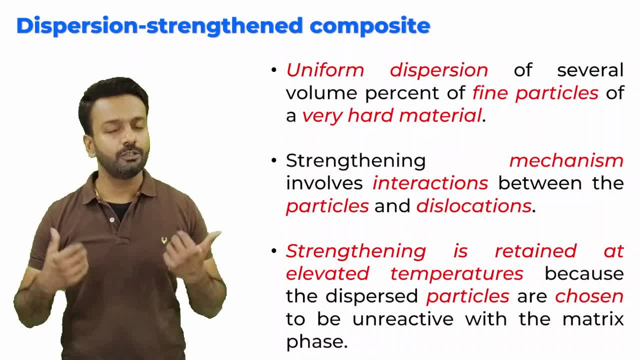 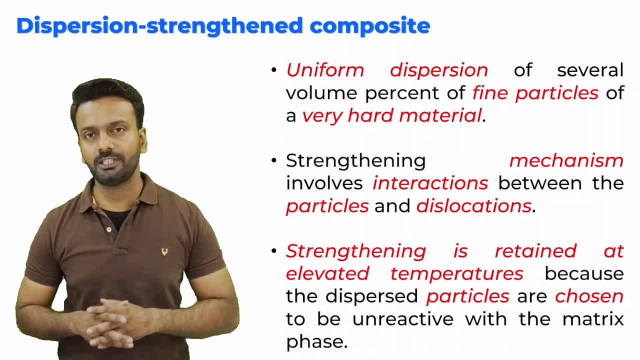 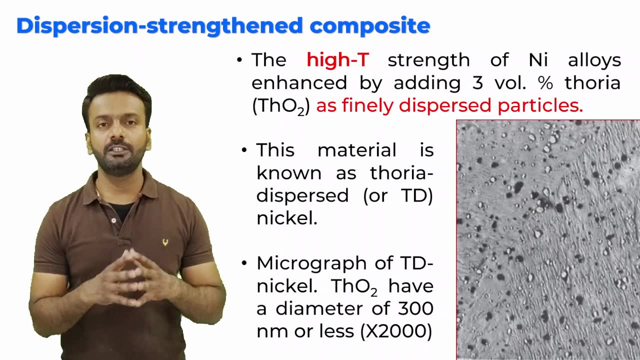 are unreactive to the matrix material and in that way you get a very strong material which is stronger at room temperature or at an elevated temperature, which is desired by your application. one example of dispersed strength in composite material is thoria dispersed nickel. here in an image you can see that high temperature nickel is mixed with around 3 percent. 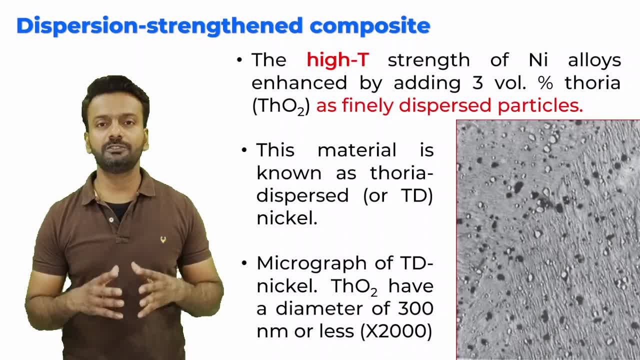 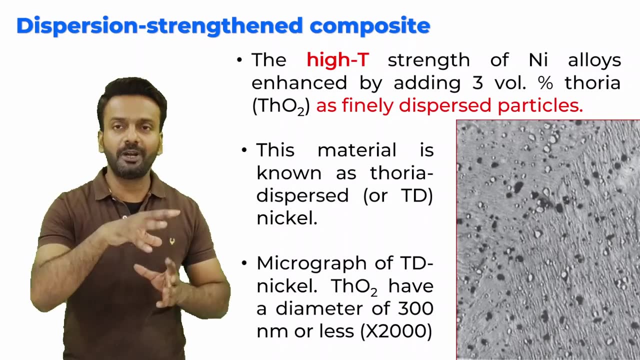 of thoria and it is called as thoria disperse. nickel and the small, small particle which are there are around 300 nanometers and they are dispersed throughout the matrix of nickel alloy. so nickel is the matrix material and these small, small thorium particles are dispersed. 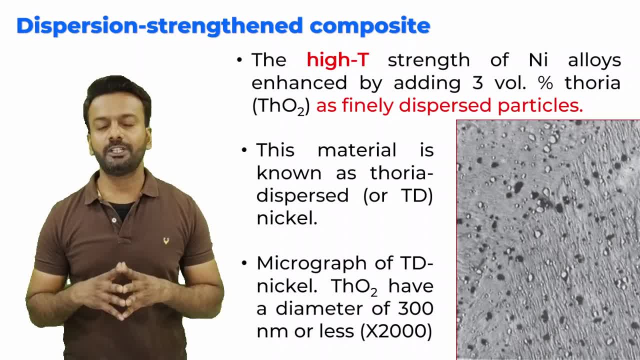 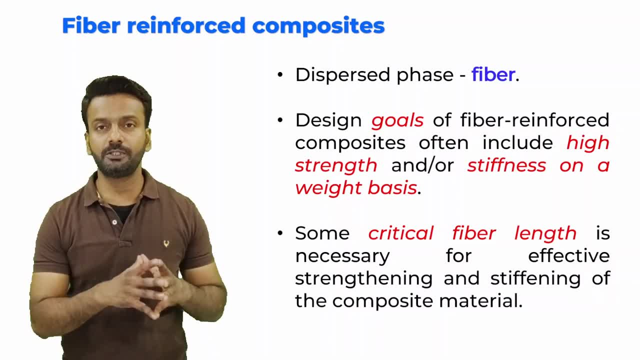 particles which are there in the matrix. finally, the composite material is called as thorium dispersed nickel. next is fiber reinforced composite material. here the dispersed phase is fiber. the design goal of fiber reinforced composite is often to include high strength and stiffness as a property of the material. so they want high strength to stiffness ratio. it. 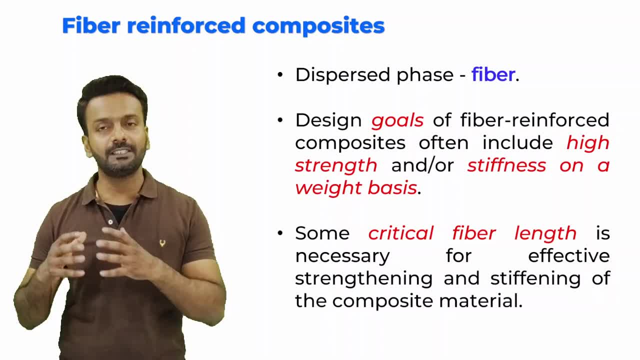 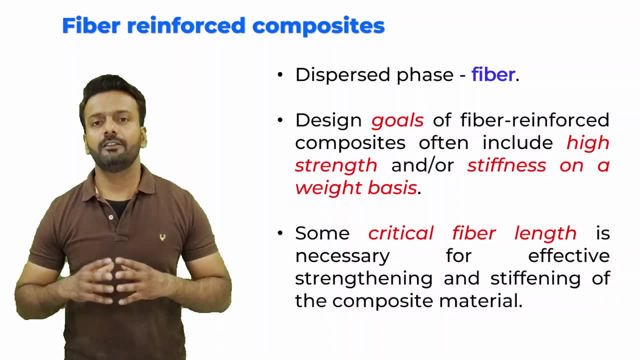 has to be very high. so the material is very strong but the weight is very less. that is the main goal when they want to make a fiber reinforced composite material also. one more important point here is that there is a critical length of fiber which we have to maintain when we are. 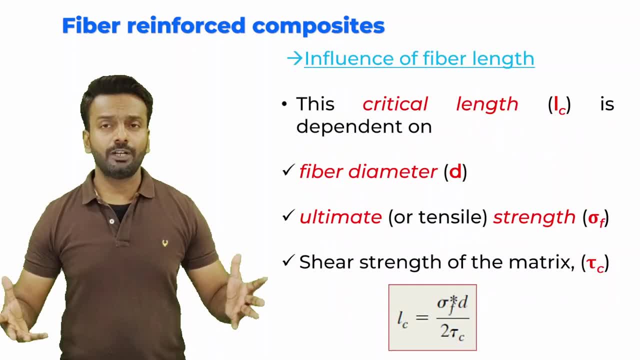 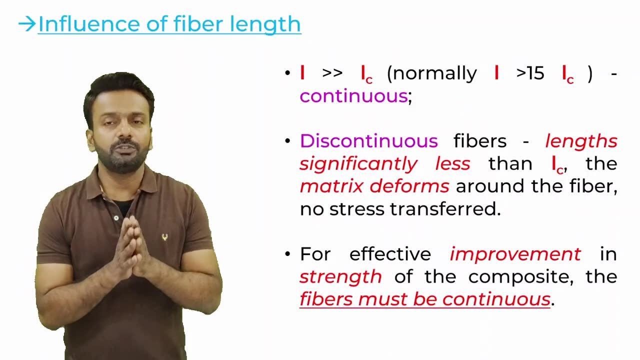 strengthening or stiffening such type of composite material. so what is this critical length, how we can determine that? and it is based on the diameter of the fiber, also the ultimate tensile strength of the fiber. so how we can classify the fiber reinforced composite material. suppose, if the 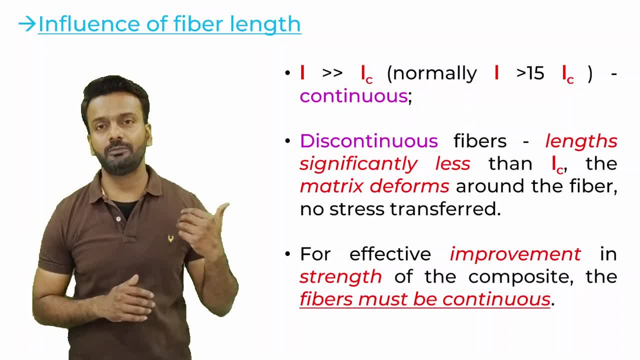 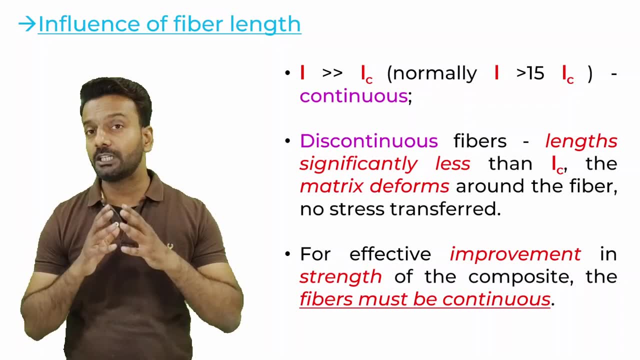 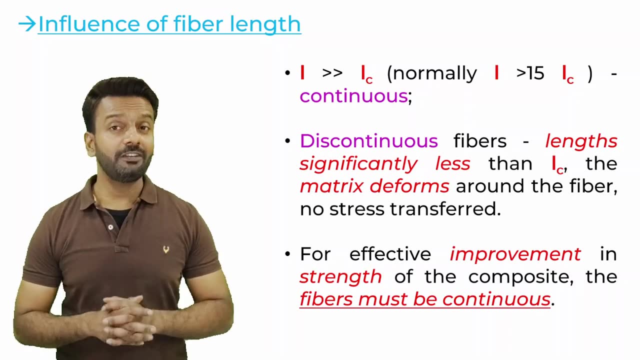 length of the fiber is very high than the critical length of the fiber generally- more than 15 times the critical length- then the fiber is said to be a continuous fiber. when the length is less than that, it is called as a discontinuous fiber. and if you want to have 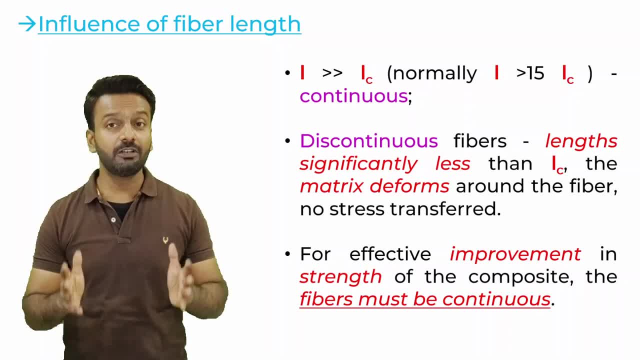 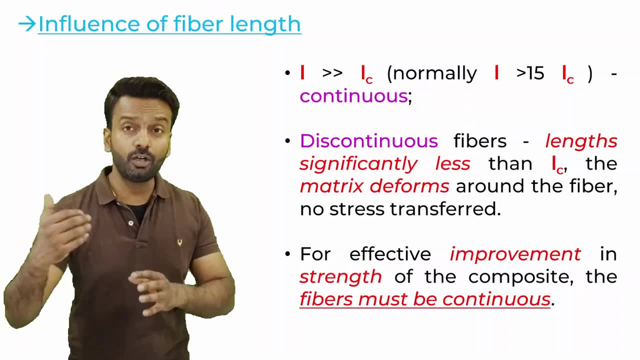 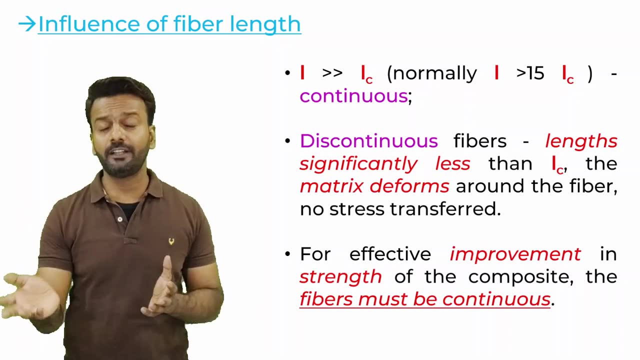 an effective improvement in the fiber. you need to have a continuous fiber, because if you have a discontinuous fiber then whatever the load is applied on the matrix, it cannot be transferred to the fiber and it becomes useless. so we can't transfer the load to the fiber from the matrix. then what is the use of the fiber which is there? so 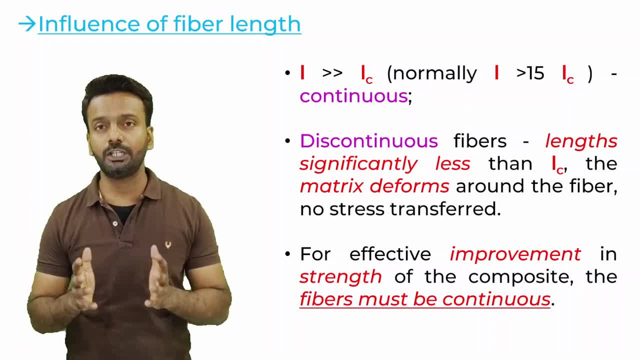 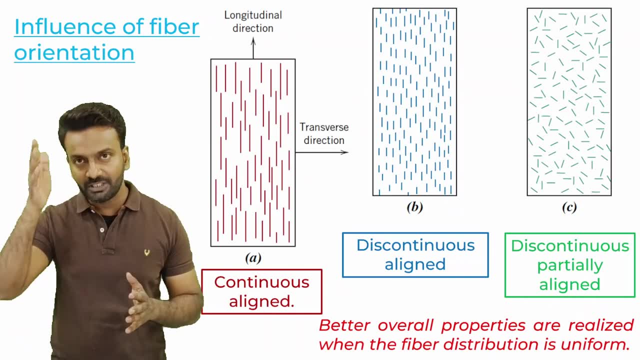 for effective strengthening of the matrix you need to have a continuous fiber. what is the influence of the fiber orientation here? in the image, you can see that you have continuous fiber which are aligned, you have discontinuous fiber which are aligned and you have discontinuous fiber which are randomly aligned. better overall properties are realized. 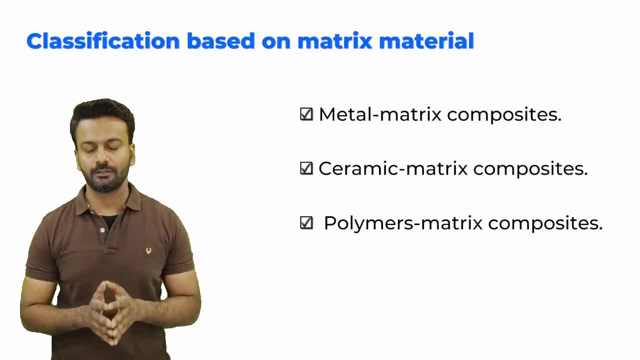 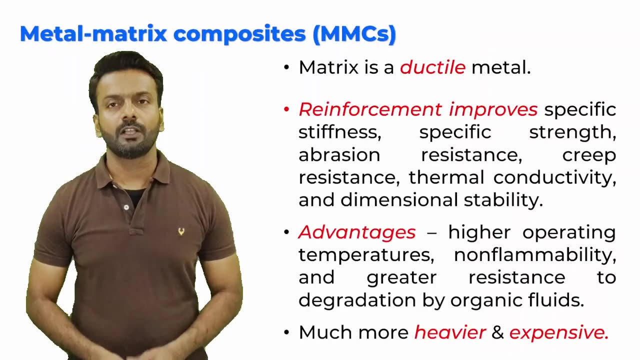 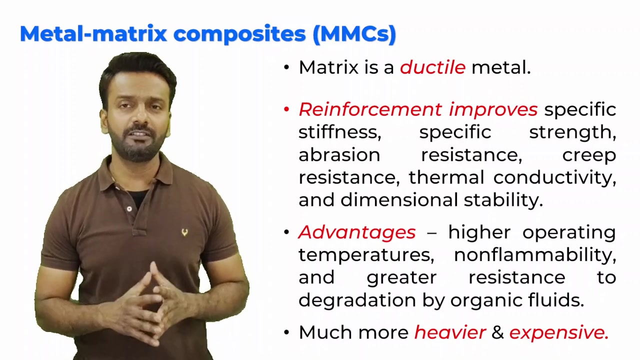 when all of these fibers are distributed uniformly. one more classification of composite material is there, which is based on the matrix material. so it can be a metal matrix composite, it can be a ceramic matrix composite or it can be a polymer matrix composite material. so in a metal matrix composite the matrix is made out of metal which is ductile, and you get certain. 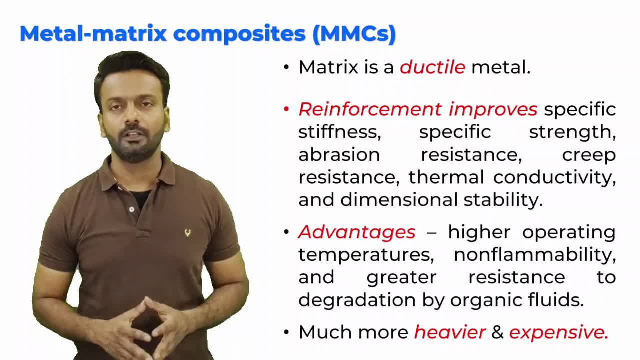 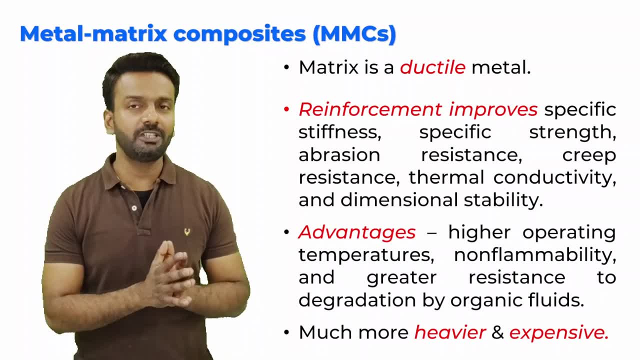 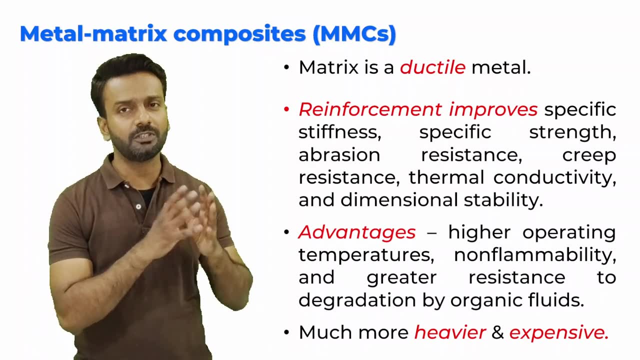 strength, you get certain different, different property you can. you get abrasion resistant property and so on. but one disadvantage here is that the matrix, the composite material, becomes really heavy and it is also very expensive. so nowadays metal matrix composite are used for certain unique application, but most of them are now replaced by ceramic matrix composite. 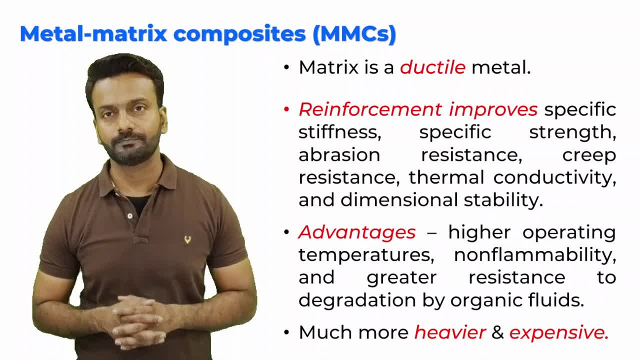 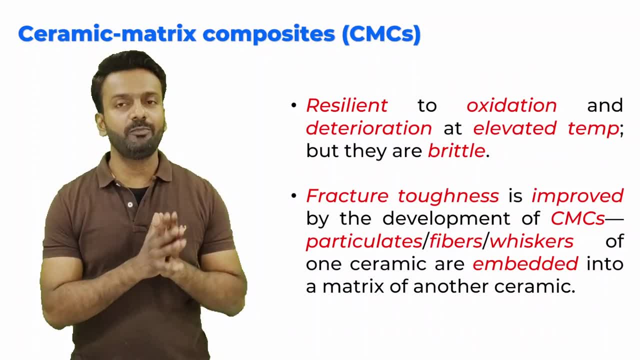 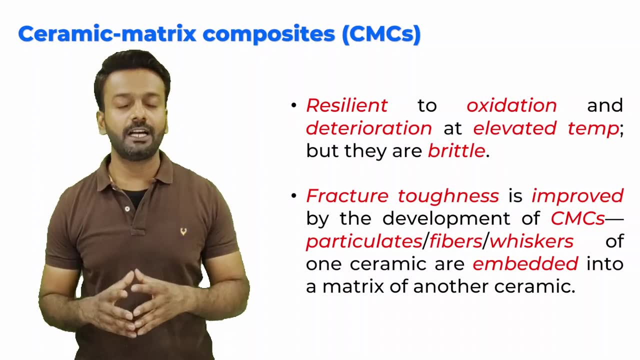 because these are much more stronger and lesser in weight. next is ceramic matrix composite. of course, the advantage of ceramic matrix composite is that that they can be operated at an elevated temperature. they are lighter in weight. but one disadvantage is that they are brittle in nature. but most of the time we can neglect this property because we get the other two properties. 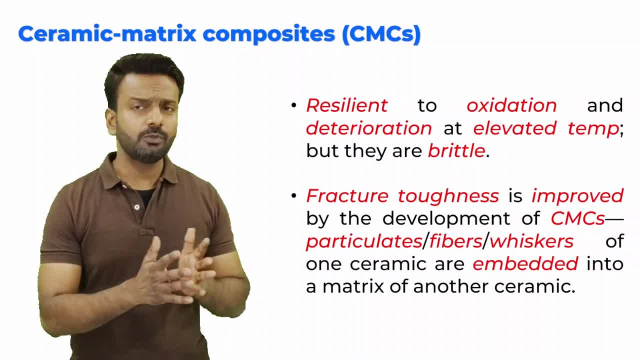 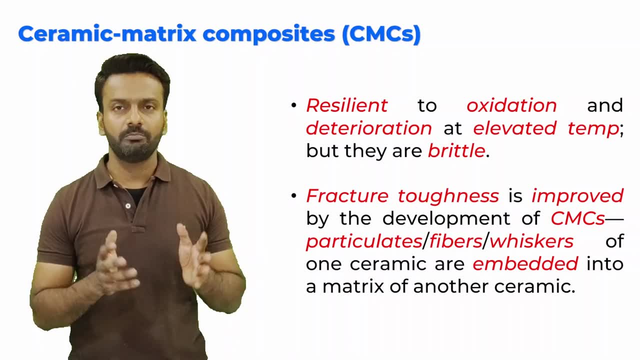 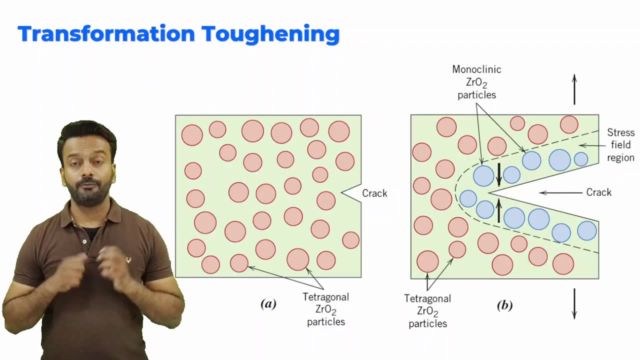 which are there in these composite material. of course, that fracture toughness of the composite material and the Hoje compound can be improved by adding small, small ceramic particles based on whisker particles or fibers to improve this fracture toughness of the composite material. fracture toughness can be improved by transformation: toughening of ceramic. 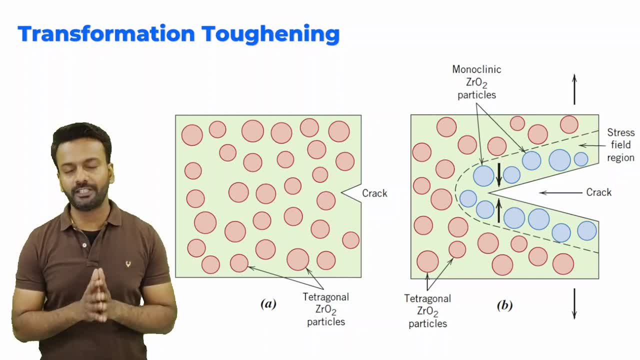 matrix composite. here you can see an example of zirconium dioxide. here small, small zirconium dioxide particles are embedded. now this ceramic matrix composite, where matrix is ceramic, the zirconia particles are also ceramic. now these are tetragonal in nature, so the crystal structure is tetragonal. now, when there is a small 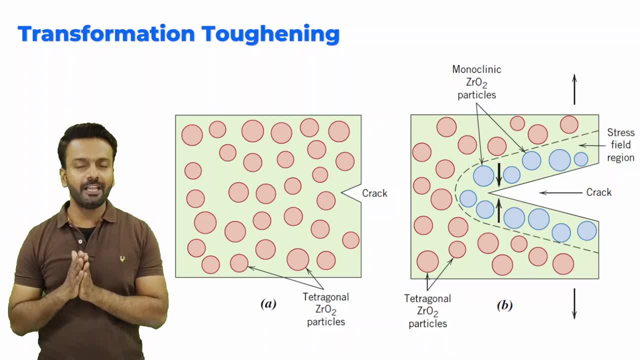 crack and when you are loading this material, the crack will try to propagate. as the crack is trying to propagate now, these tetragonal particle will transform into zirconia particle. so the structure is different now. because of the difference in structure here, the crack will be arrested. 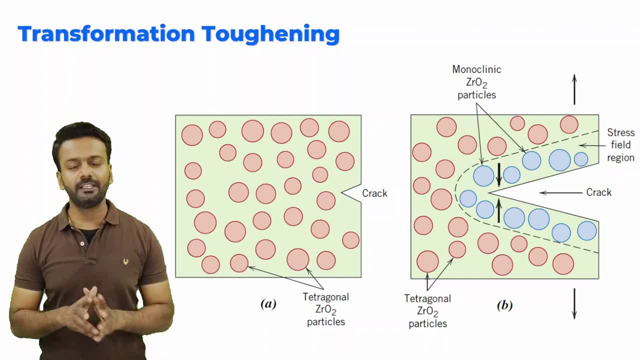 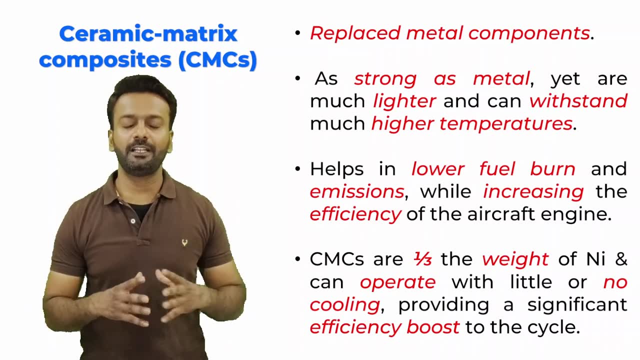 it cannot go further. because of this the material will not break, the crack will not propagate. as i told earlier, the ceramic matrix composite have replaced the metal matrix composite mainly because they are lighter in weight. they can be operated at higher temperature. main application of ceramic matrix composite is in airplane engine, so the engines are made out of. 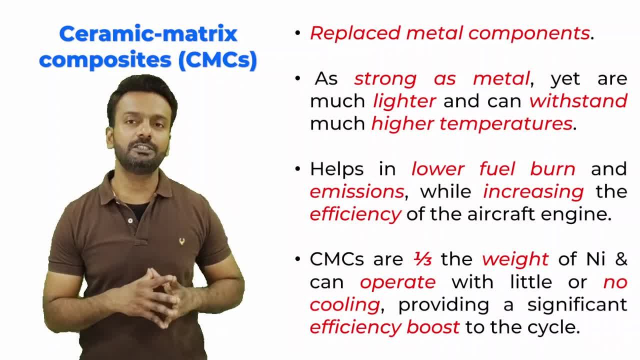 cmcs- where they have replaced the original ceramic matrix composite with the ceramic matrix composite which is the ceramic original engine- which were made out of nickel alloy. so these cmcs are one-third of the weight of the nickel alloys which were used earlier. also, they can be operated with no or very little cooling. 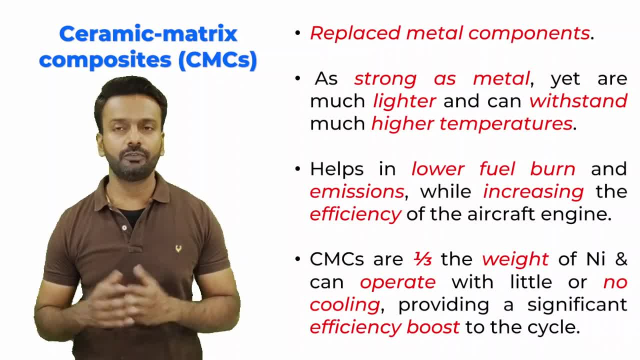 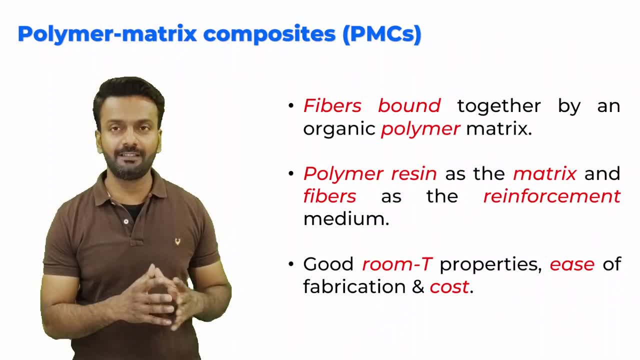 and this gives a significant boost in efficiency of the aircraft engine. next is the polymer matrix composite. so here the matrix material is polymer resin and you are putting some fiber inside, making a polymer matrix composite. the the polymer matrix composite are very cheaper to make. also the ease of fabrication is there. but one disadvantage is that 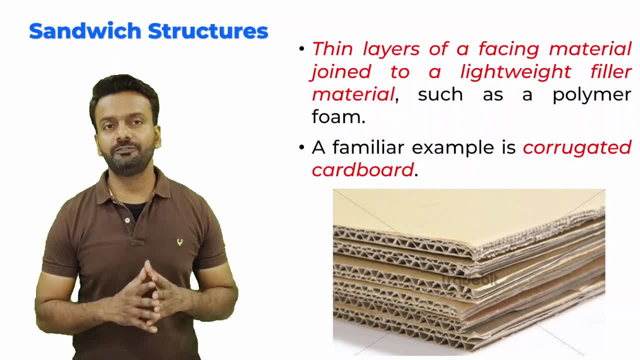 they cannot be operated at a higher temperature. next classification is a sandwich structure. a sandwich structure is nothing but some facing material. is there like two layers, and in between these layers you are filling in some filler material. that filler material can be used based on different property, like sound, absorption property and so on. one familiar example of a sandwich: 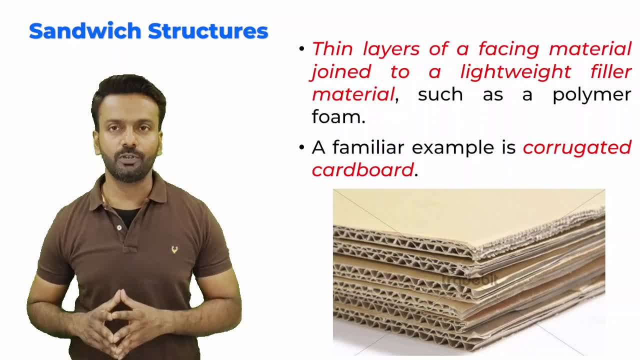 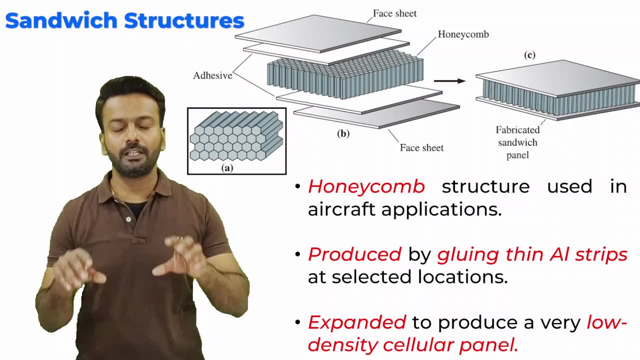 structure is nothing but a corrugated cardboard. another example of sandwich structure is the honeycomb structure. here in the honeycomb structure, if you see in the image, you can see that aluminum strips are there. aluminum strips are glued together and then there is one facing material. 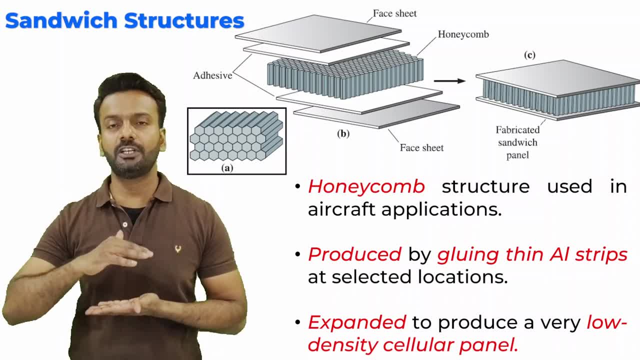 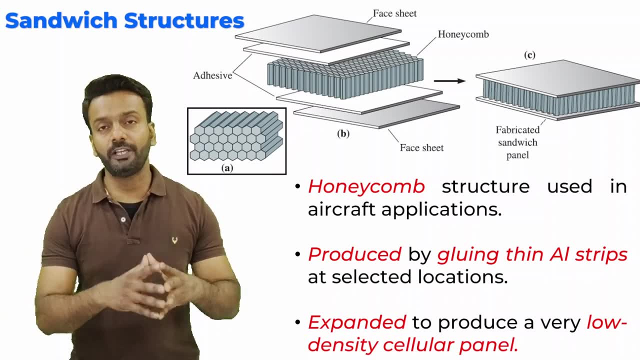 which is there, which is supporting these aluminum strips which are there, and you are forming a sandwich structure. honeycomb structures are used in aircraft application where you want to reduce the weight of the material which is used in the aircraft. so, for example, if you have a sandwich. 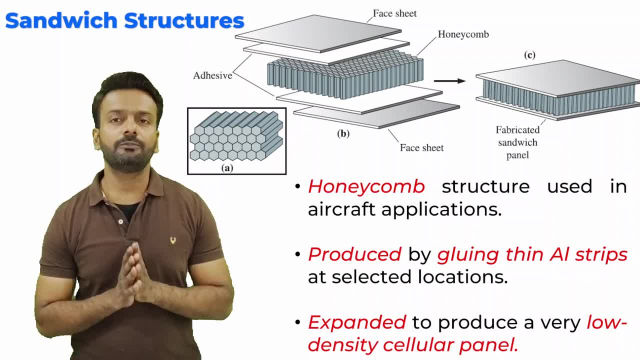 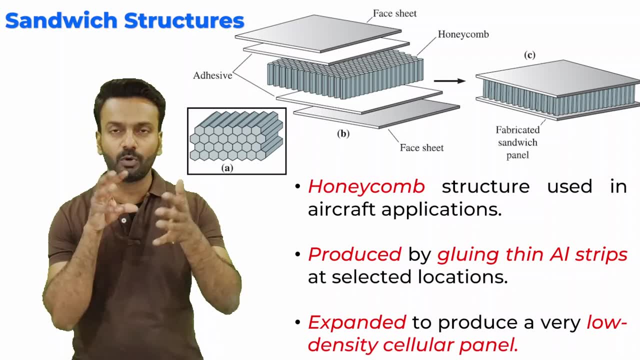 structure. you can make a sandwich structure using this sandwich structure and then you can make a sandwich structure from these panels, and this sandwich structure is made of different panels which are there in the aircraft. they are now made out of these sandwich structure and, if you want to, 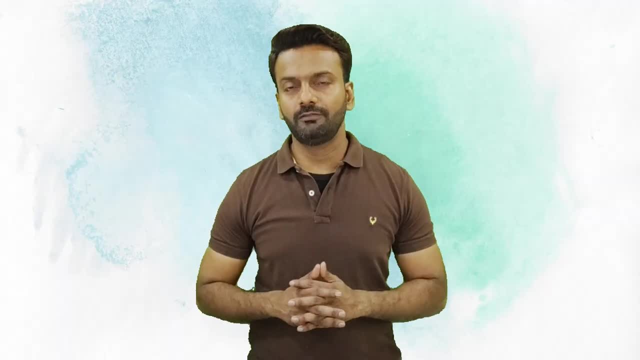 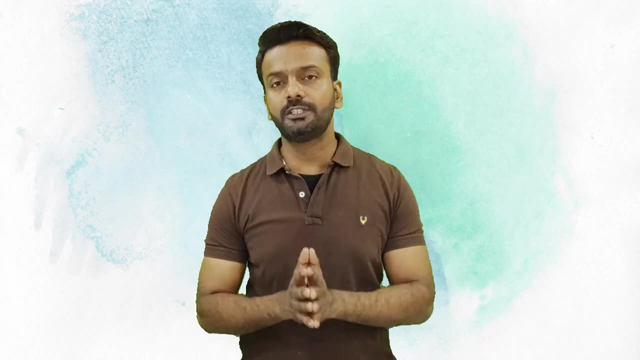 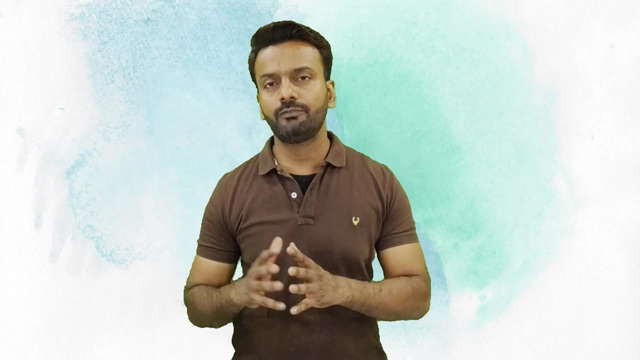 make them sound proof. you are putting some foam inside these small small gaps which are there and making a good sound proof sandwich structure. so let us summarize what we have learned in this lecture. today we have classified the composite material- nano composite- we will discuss later on. in particle reinforced composite we saw large particles and